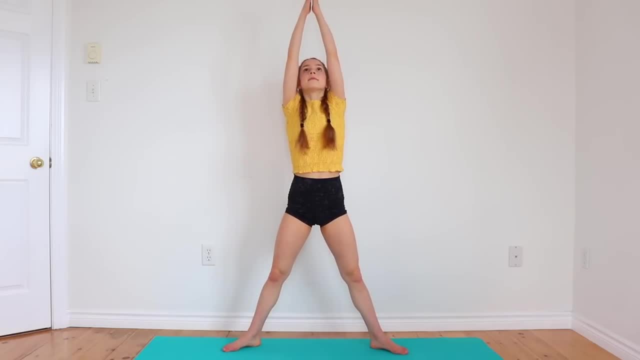 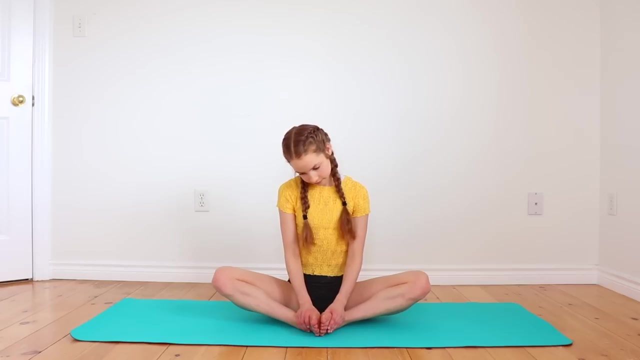 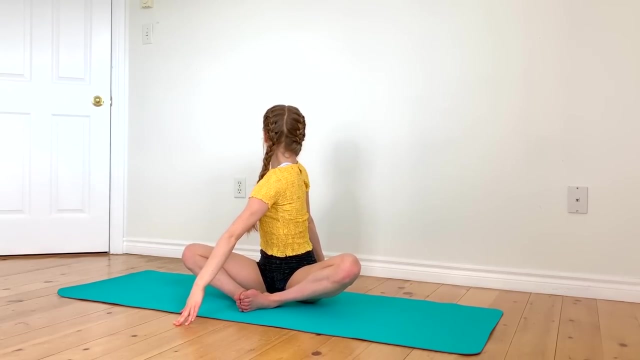 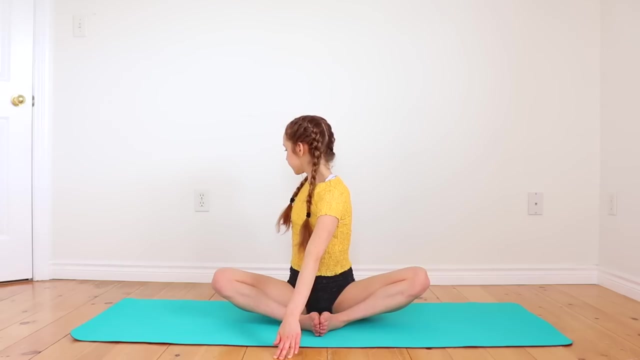 Now sit down in a butterfly stretch. Now we're going to do some basic stretches while staying in this butterfly sit, starting with neck circles. Now go ahead and switch directions, And now we're going to reach up and stretch. And now twist your body to one side. 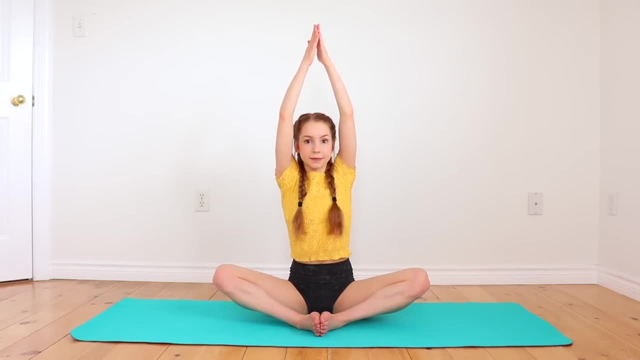 Reach up again, and we're going to repeat that on the other side. Next, bring one arm across your body and pull it towards your chest Switch to stretch out your other arm. And now take that same arm and pull it over your head to stretch out your shoulder. 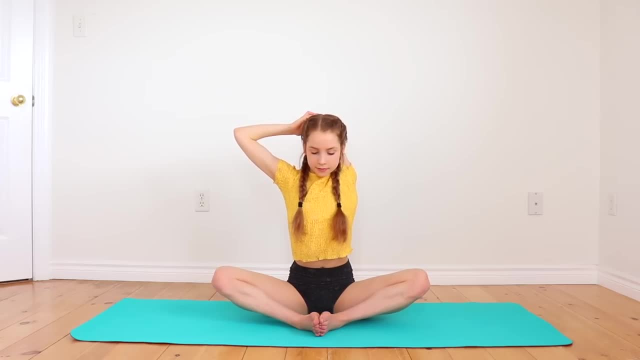 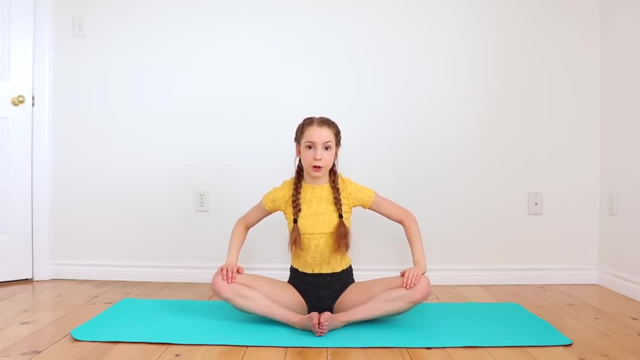 Good, Good, Good, Good, Good to the ground, if you can. so you want to push it enough so that you feel a good stretch, but you don't want this to be painful, so just push it as far down as you can to feel a stretch, but no pain. 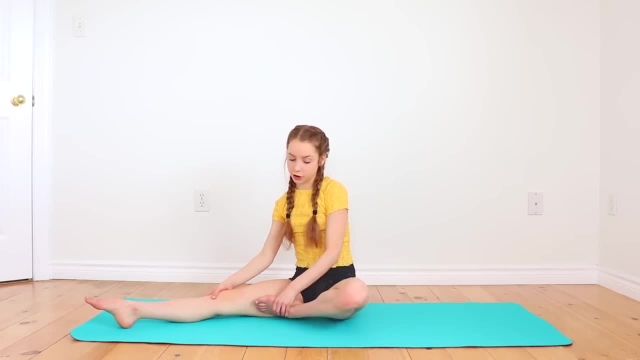 now straighten up one leg and pull the other leg to your inner thigh, and we're going to reach up and then reach forward, trying to grab onto your ankle. if you can, if you're up here, that's fine too. as long as you feel a stretch in your hamstring, or if you. 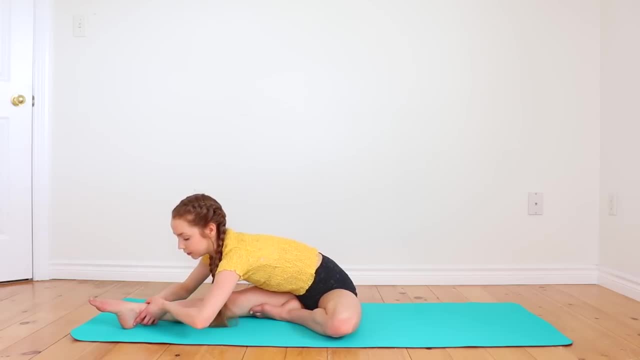 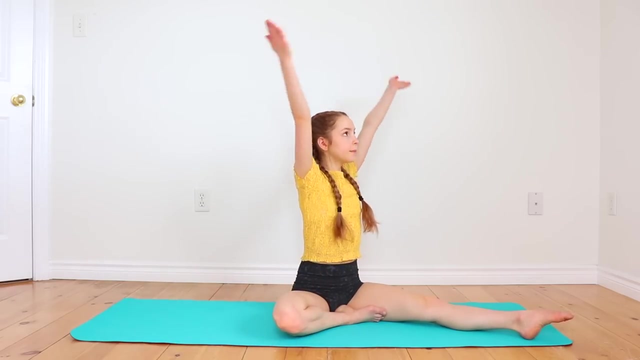 don't feel a stretch grabbing onto your ankle, you can try to pull your chest even further, but for now, right here, is probably going to be good for most of you. now we're going to switch to do that on the other leg, so reach up and reach forward trying to grab your ankle or, like i said, you can go even further if you don't feel a stretch. 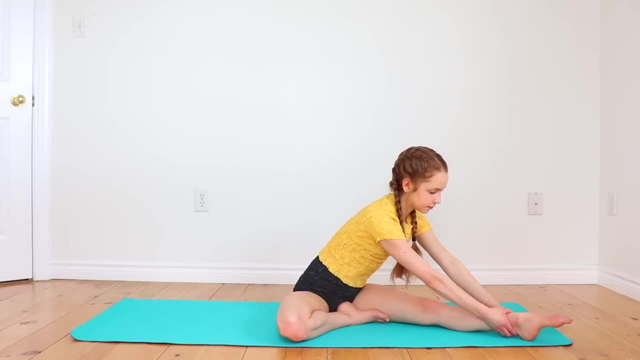 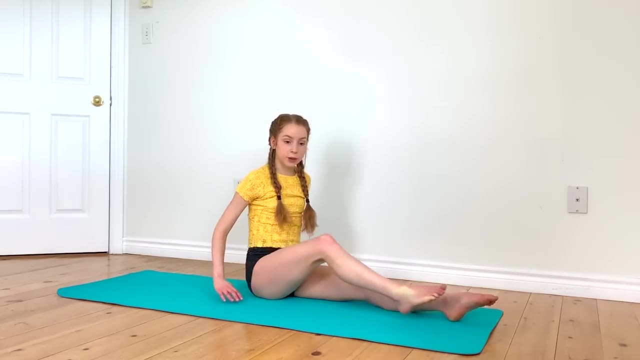 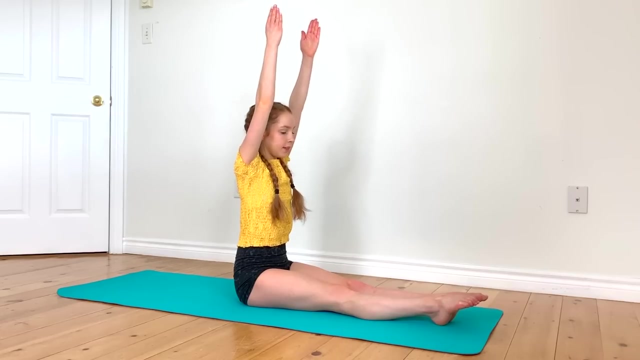 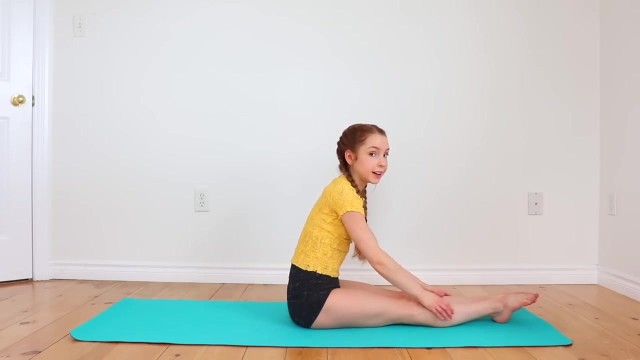 now straightening out both legs in front of you to do a pike stretch. so we're going to reach up again and this time reach forward, trying to grab onto your toes if you can. if you can, then just reach forward onto your knees as long as you feel that stretch. 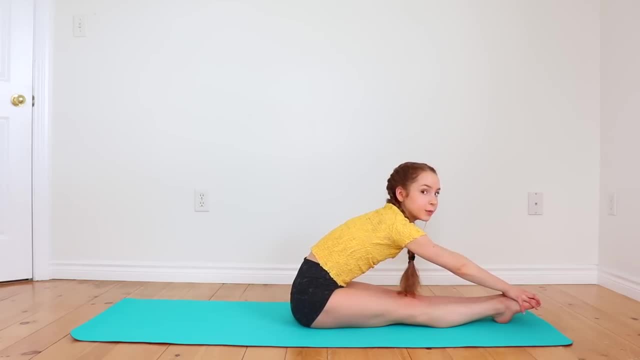 but if you can reach forward to your toes and try to point them towards you, but if you can reach forward to your toes and try to point them towards you, the ground to get a good stretch in your feet as well. again, you can always modify the stretch to go further down, to get more of a 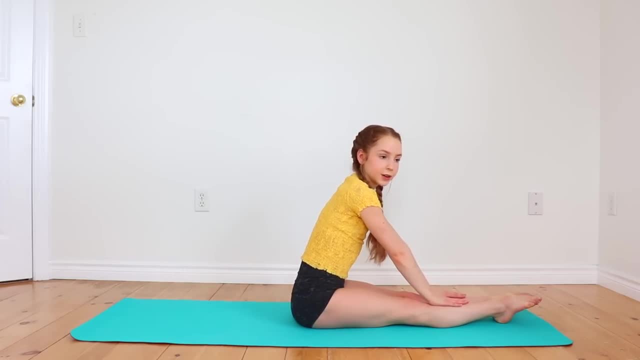 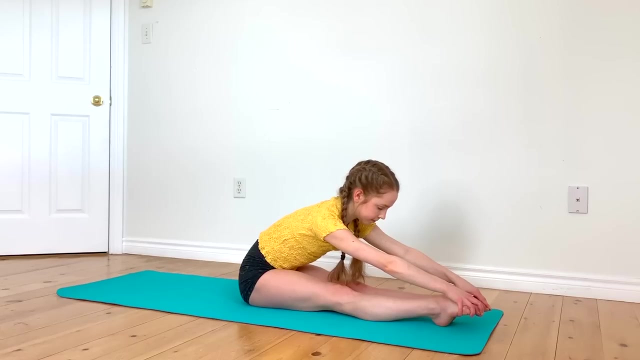 stretch. or, like i said earlier, you can just stretch. or, like i said earlier, you can just stretch. or, like i said earlier, you can just stay right here. just stay right here. we're going to repeat that same stretch, except this time with your feet. we're going to repeat that same stretch, except this time with your feet. 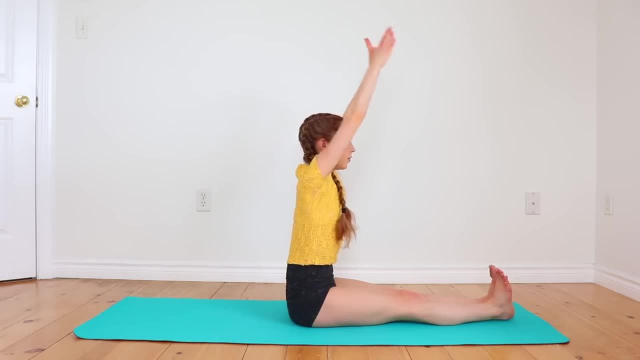 flex. so reach up again and reach forward, trying to pull your toes towards you to get an even deeper stretch in your hamstrings. feel your water. feel your water. If you don't feel that deep of a stretch, you can always bend your elbows, or if you. 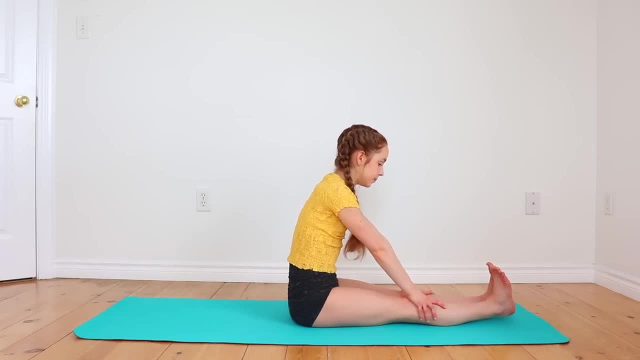 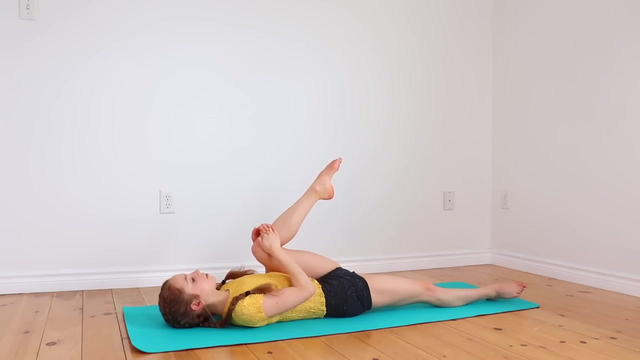 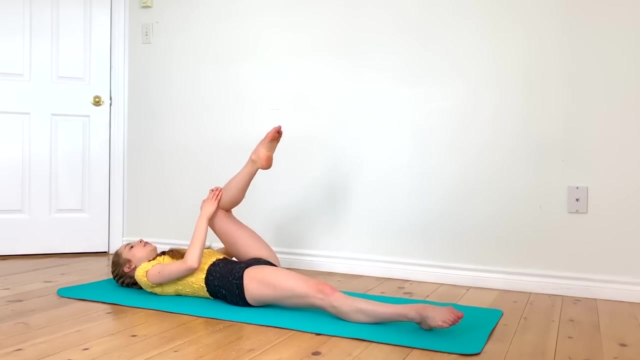 can't reach your toes, just flex your feet and grab onto your knees. You can now relax your feet and we're going to lay back on our back and then, once you're down here, bring your knee to your chest. Now try to straighten your leg, trying to get your foot up towards the ceiling, or if 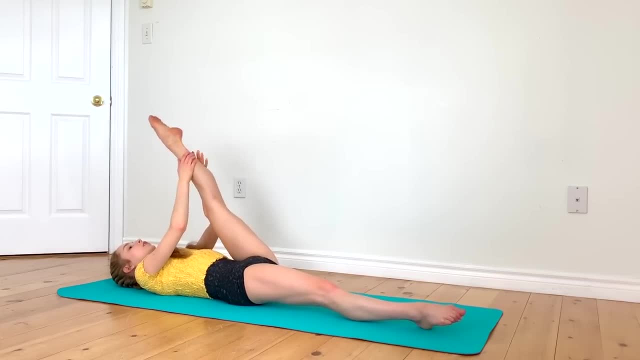 you don't feel stretched, you can pull it even further, but for a beginner you're most likely going to be around this level. Now you can bend that leg again and pull it across your body, trying to leave both shoulders on the ground. 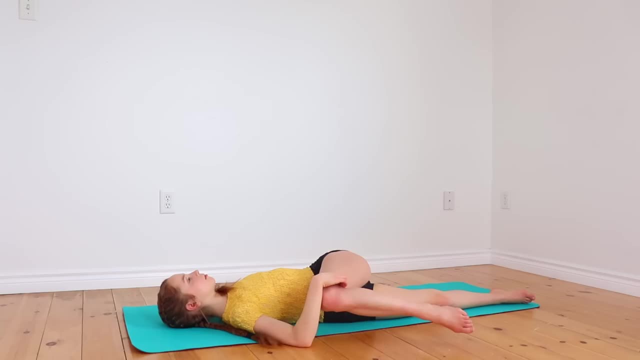 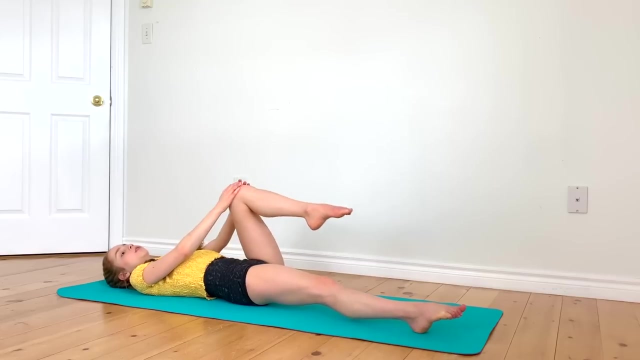 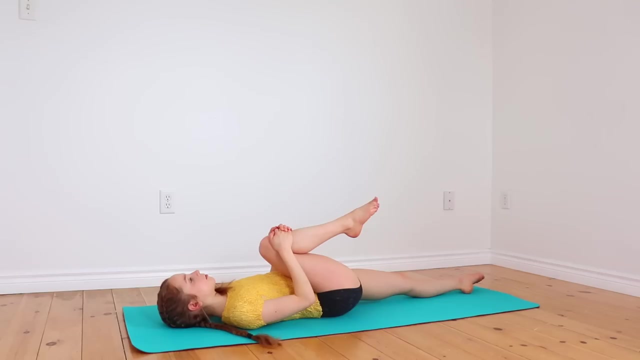 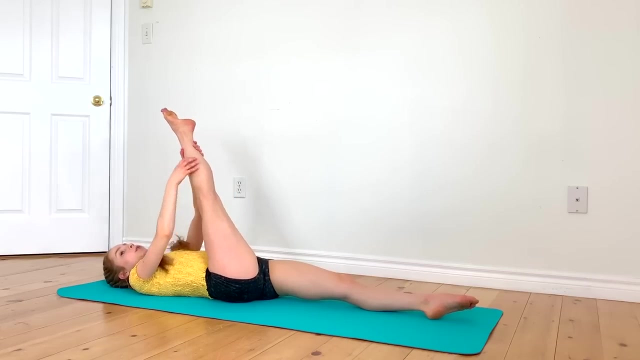 Bring it back up to center and we're going to repeat those three stretches on the other leg. So start with pulling your knee to your chest And now straighten it out to whatever height you can. so you might be here or you might. 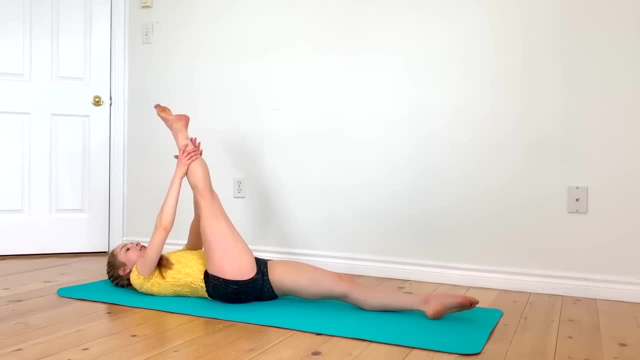 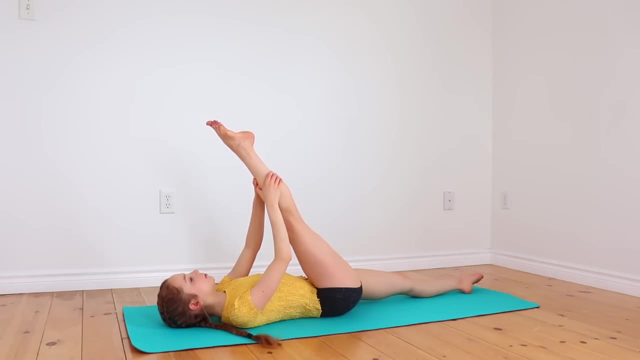 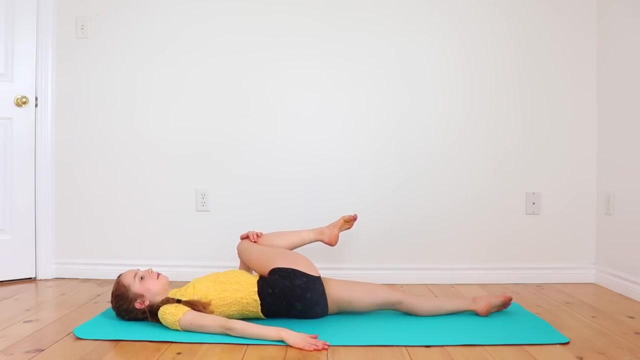 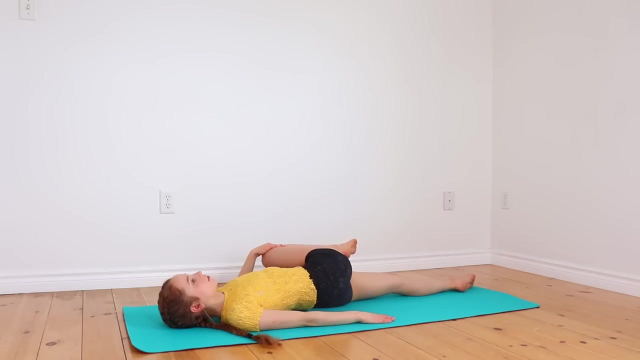 be even closer to your face. It really just depends on what level of flexibility you're starting at. And now bend that leg in and pull it across your body. Remember to leave both shoulders on the ground. Now we're going to bend our legs. 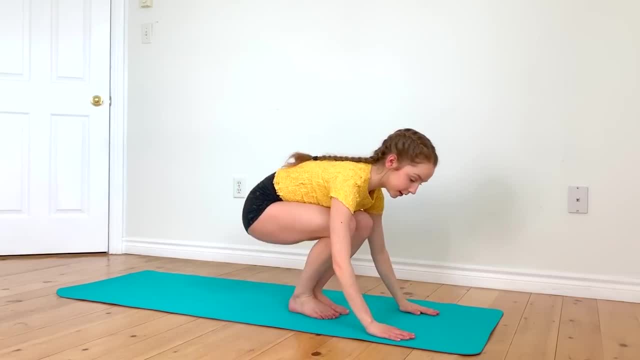 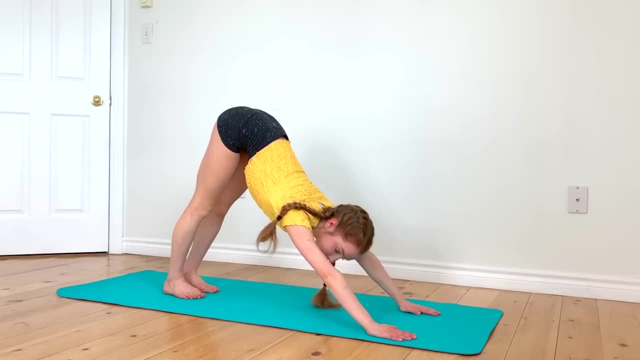 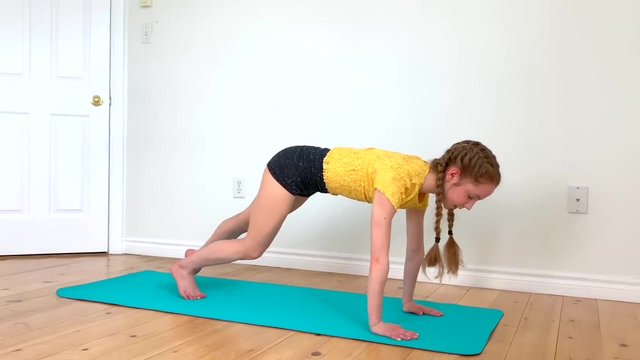 You can now sit back up and relax, and we're going to go up into a downward dog position, So in this you should be trying to push your heels towards the ground and your chest back. Good, From here, push your hips towards the ground. 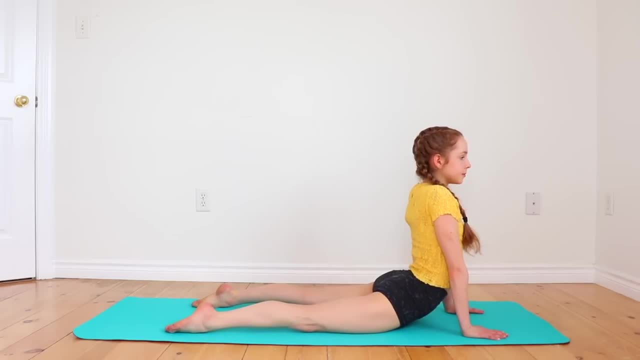 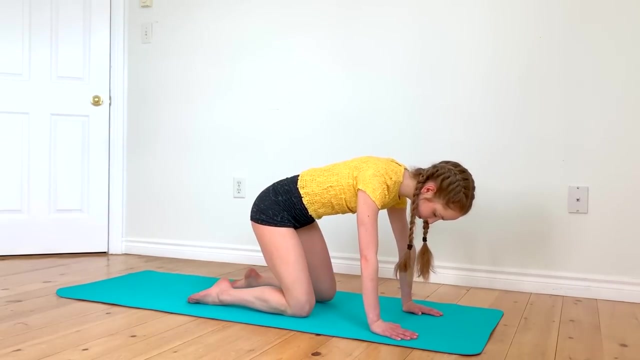 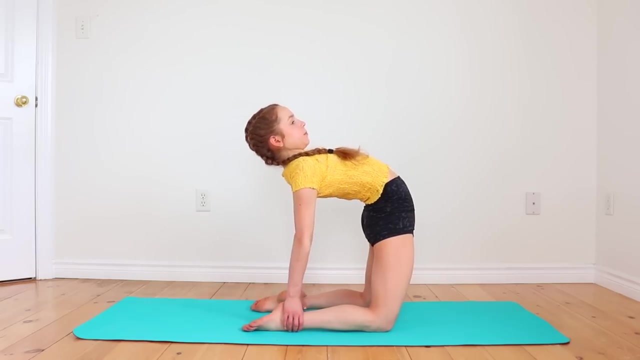 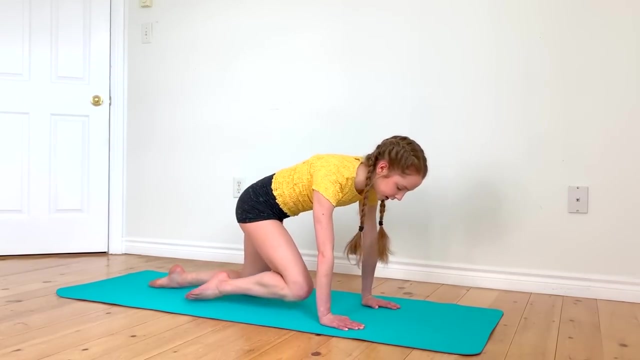 into a seal stretch to stretch out your back And now go up onto your knees and we're going to arch back and, if you can, try to grab onto your ankles. Now we're going to go onto our hands and knees and we're going to start by arching back to 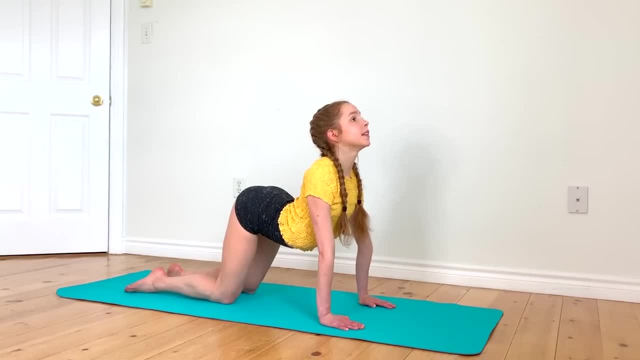 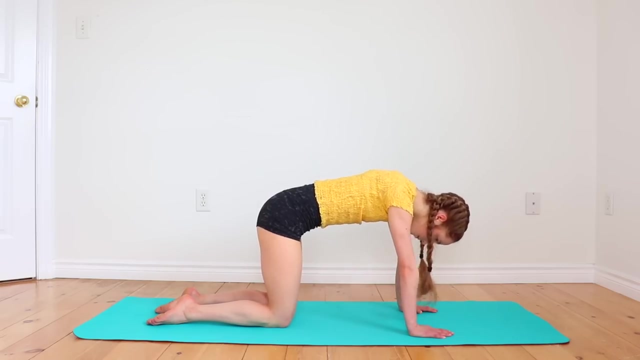 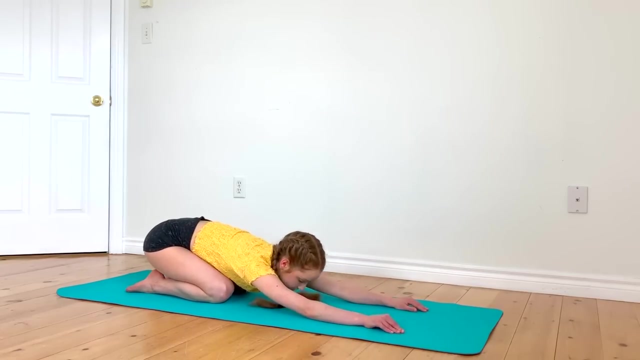 stretch out your back again and then contract. We're going to do that four more times And to finish off this stretching routine, we're just going to go down into a child's pose And that's it for this stretching routine. so I hope it helps you improve your flexibility. 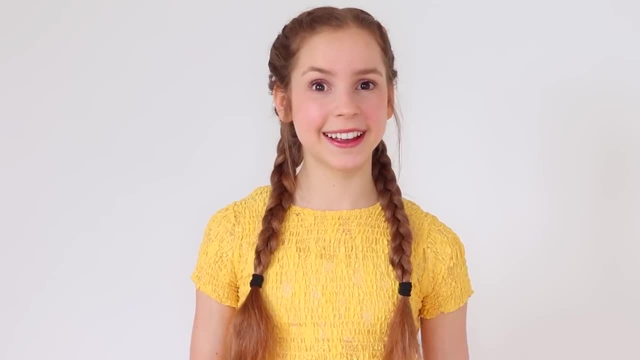 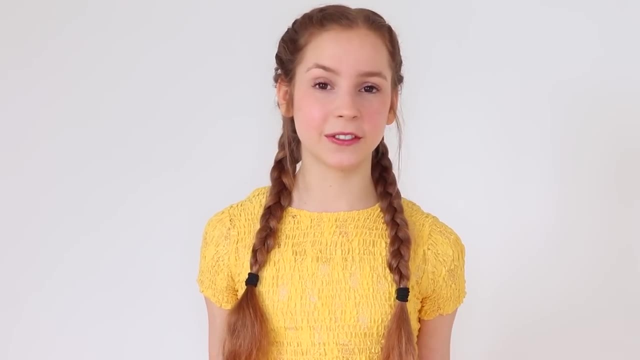 If you know of someone else who's trying to improve their flexibility as well, definitely share this routine with them. or if you would like a more advanced routine, I have lots more stretching routines on my channel and I'll link a few in the description below. 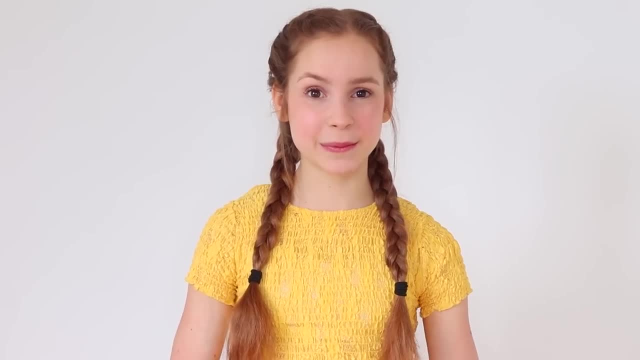 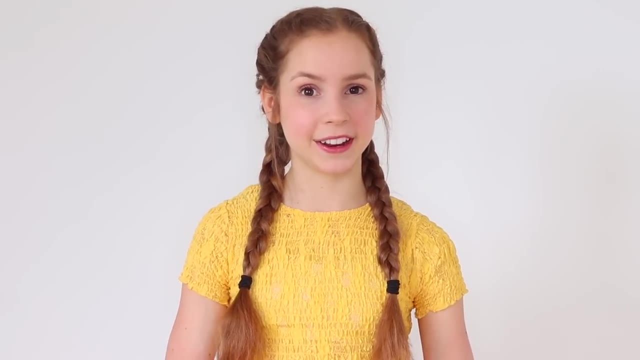 Like always, I'd really appreciate it if you could give this video a thumbs up and also subscribe to my channel as well as click on the notification bell so you get notified whenever I upload any new videos. Bye guys, Bye guys.